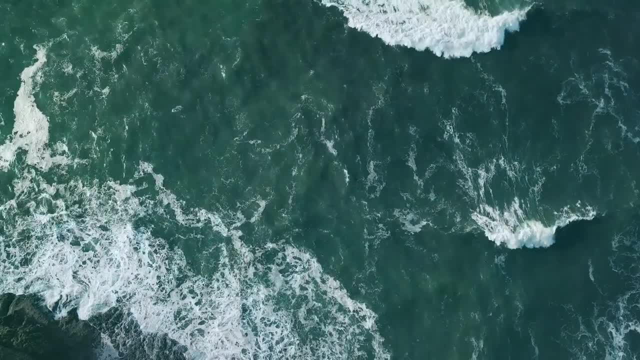 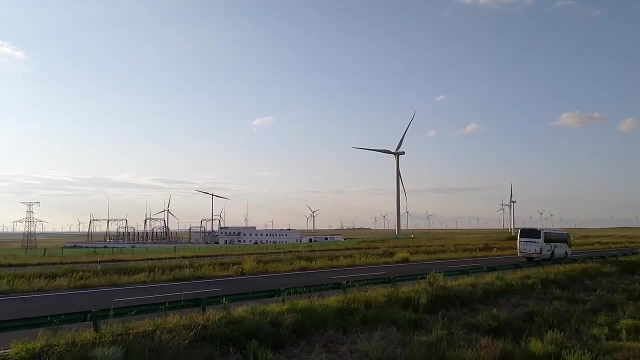 Now let's dive deeper into each of the three fundamental forces described by the standard model. The electromagnetic force is responsible for the interaction between charged particles such as electrons and protons. This force is described by the theory of electromagnetism, which was first proposed in the 19th century. The electromagnetic force is responsible for the 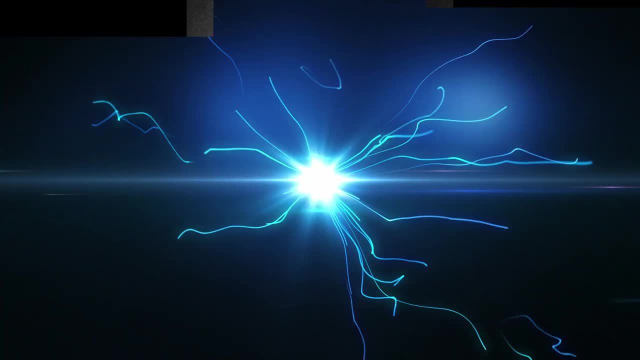 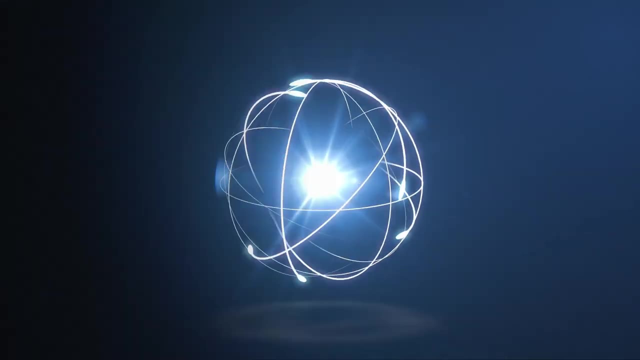 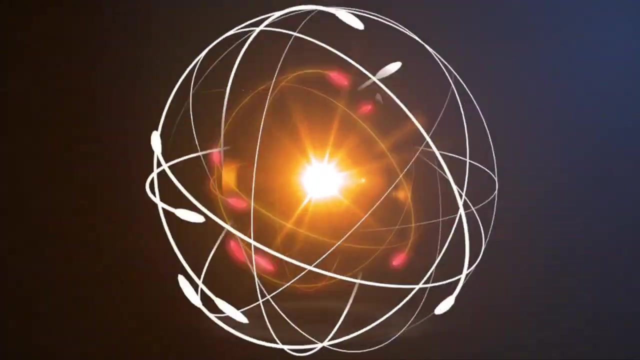 interaction between charged particles such as electrons and protons. The strong nuclear force is responsible for holding the nucleus of an atom together. This force is described by the theory of quantum chromodynamics. QCD describes the interaction between quarks, which are the 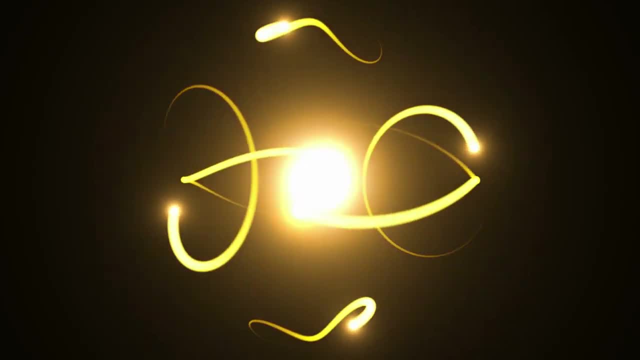 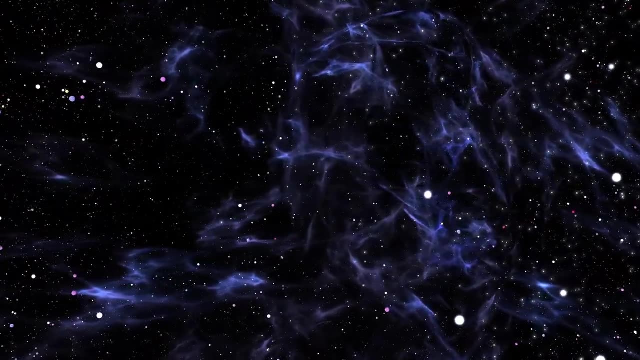 particles that make up protons and neutrons. The strong nuclear force is mediated by particles called gluons. They bind quarks together and they form a strong nuclear force. The strong nuclear force is the building blocks of atomic nuclei. Without the strong nuclear force, atoms would not be stable. 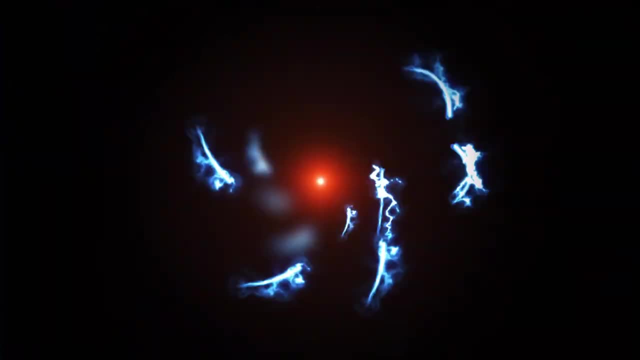 and the universe as we know it would not exist. The weak nuclear force is responsible for certain types of radioactive decay. This force is described by the theory of electroweak interaction, which was developed in the 1970s by Sheldon Glashow, Abdus Salam and Steven Weinberg. 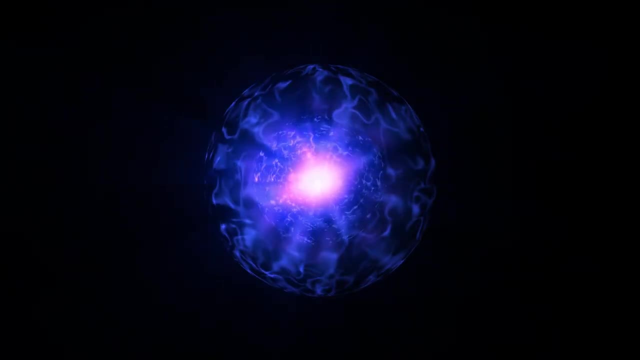 The theory of electroweak interaction describes how the weak nuclear force and the electromagnetic force are interrelated. The weak nuclear force is responsible for the interaction between quarks. Now let's talk about some of the latest developments in the Standard Model. 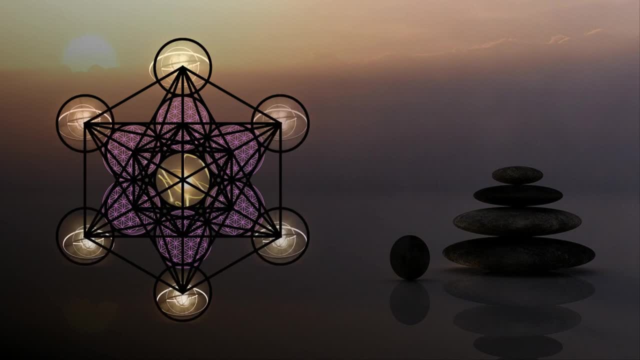 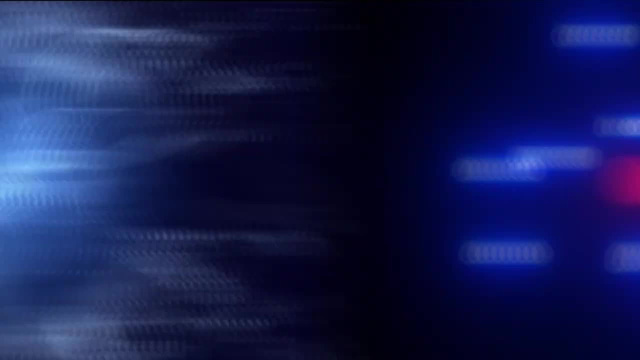 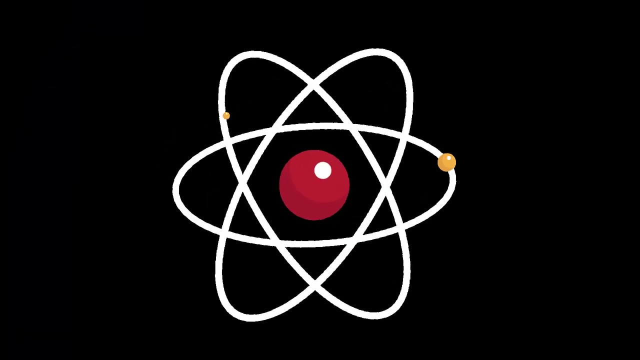 One of the biggest challenges in the Standard Model is the hierarchy problem. The hierarchy problem refers to the large difference in energy scales between the weak nuclear force and gravity. In the Standard Model, the energy scale of the weak nuclear force is much smaller than the energy scale of gravity. This means that there must be some unknown. 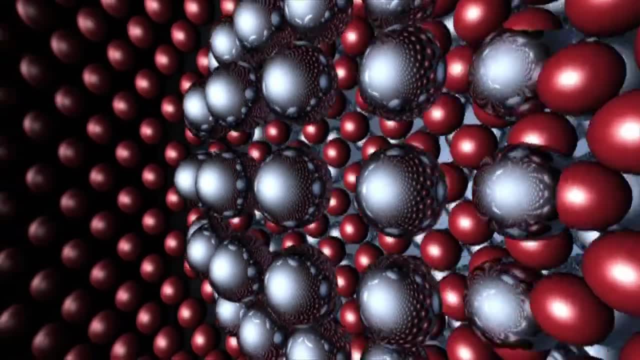 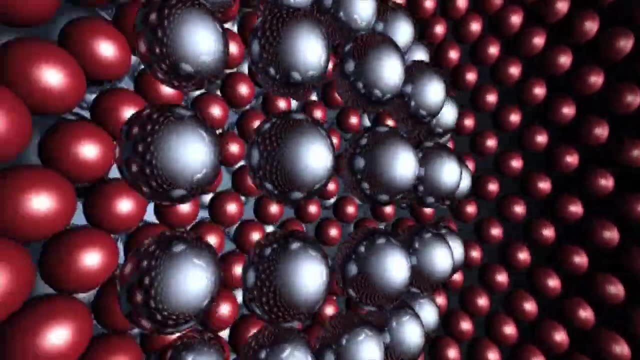 mechanism that keeps the two scales separate. Many physicists believe that this mechanism could be related to the discovery of supersymmetry. Supersymmetry is a theoretical concept that predicts the existence of a new set of particles that are related to the particles in the standard. 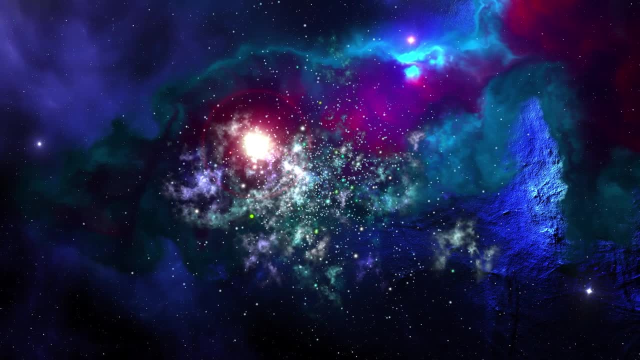 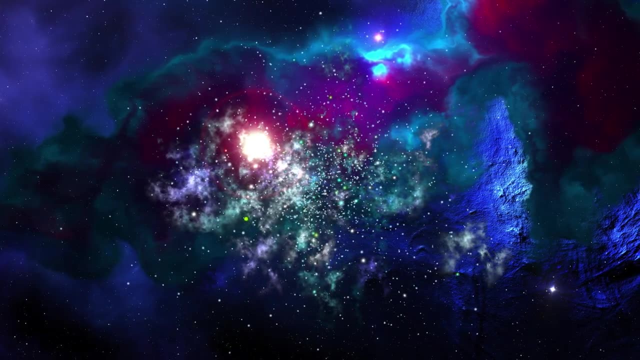 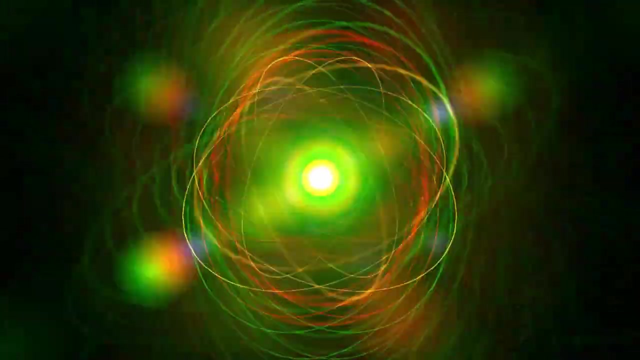 model, These particles are known as supersymmetric particles or sparticles. Supersymmetry would provide a natural explanation for the hierarchy problem, as it would introduce a new symmetry between fermions and bosons. Another recent development in the standard model is the discovery of neutrino oscillation. Neutrinos are particles that have no electric charge and very 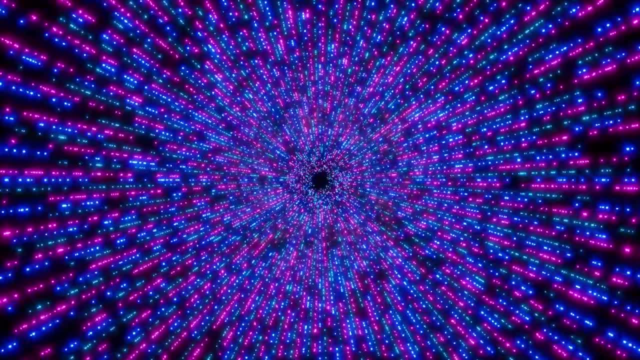 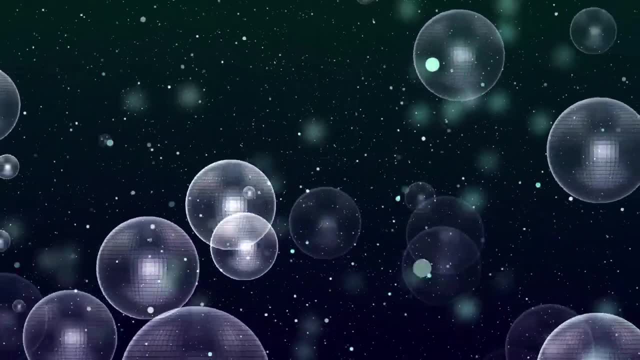 little mass. Neutrino oscillation refers to the phenomenon where neutrinos change from one flavor to another as they travel through space. There are three known types or flavors of neutrinos called electron, muon and tau neutrinos. As neutrinos travel through space, they can undergo 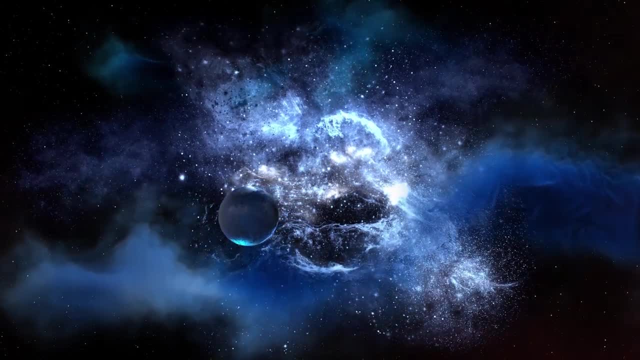 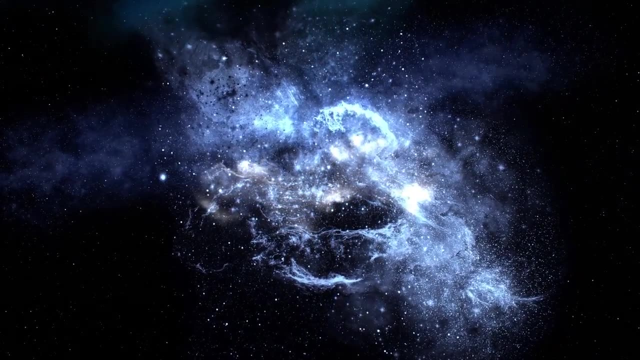 quantum mechanical interference causing them to change their flavor. This means that a neutrino that was initially produced as an electron neutrino can change into a muon or tau neutrino, and vice versa. This discovery was made in the late 1990s. 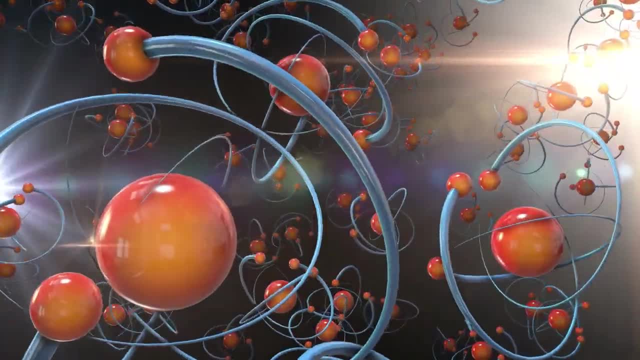 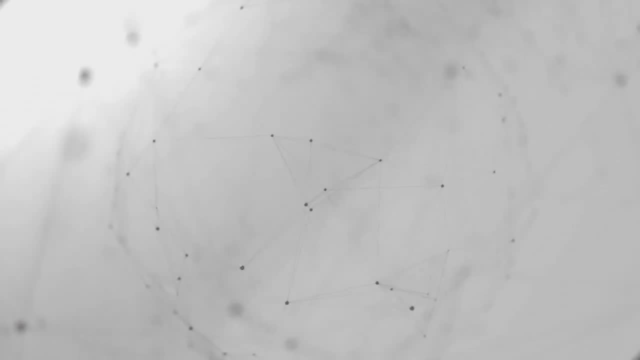 and early 2000s, and it confirmed the existence of neutrino masses which were not predicted by the standard model. The discovery of neutrino oscillation has led to further research into the properties of neutrinos, including their mass hierarchy and whether or not they violate. 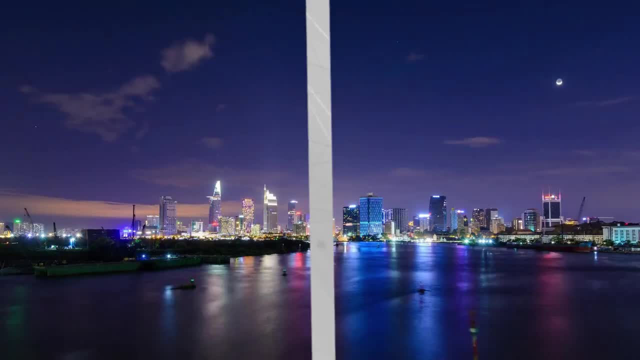 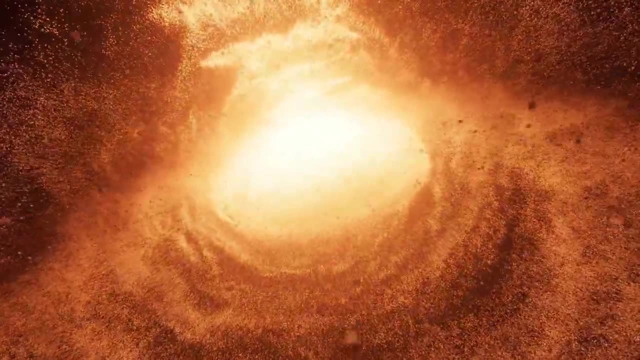 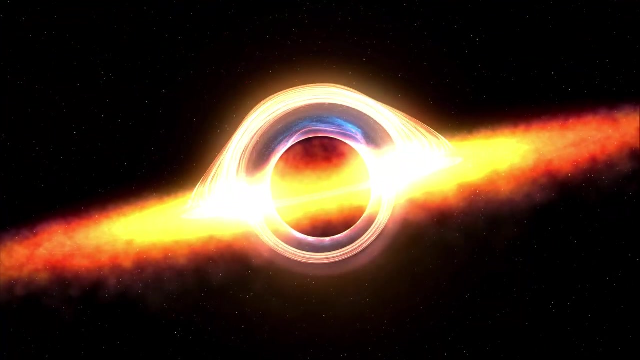 a fundamental law of physics known as CP symmetry. These questions are being studied by a number of experimental collaborations around the world. In addition to these developments, there are also ongoing efforts to unify the forces described by the standard model with gravity. This is known as the problem of quantum gravity, and it remains one. 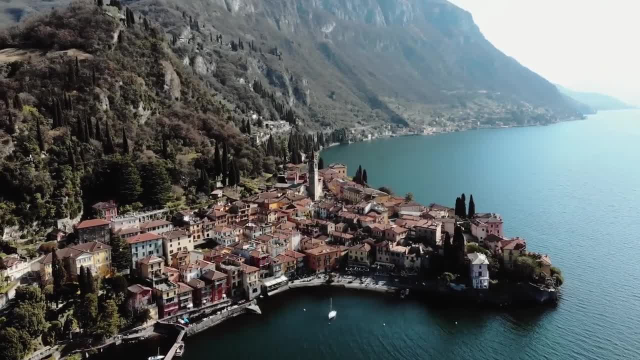 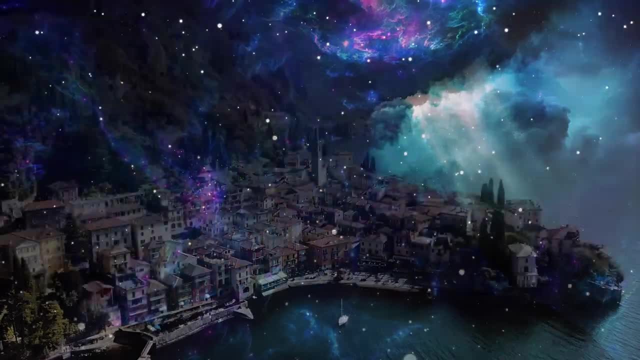 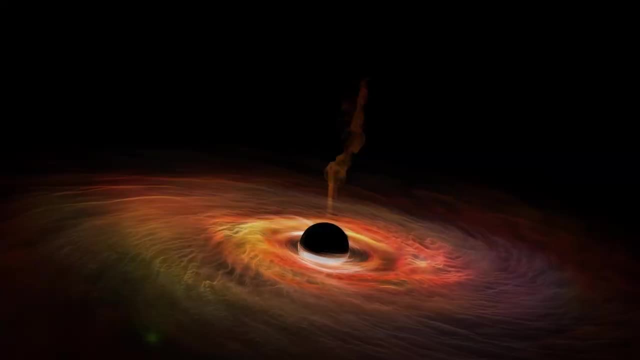 of the biggest challenges in physics. Many physicists believe that a theory of quantum gravity will require the development of a new theoretical framework that goes beyond the standard model. Overall, the standard model is an incredibly successful theory that has been rigorously tested through experiments and observations. However, there are still many. 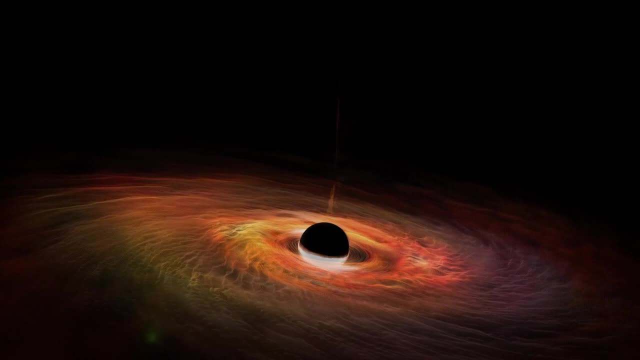 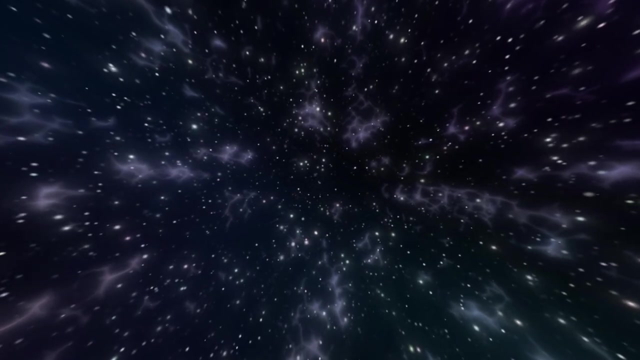 questions that remain unanswered, and the search for new physics beyond the standard model continues. So that was all for this video. I hope it has given you a better understanding of the standard model and its place in our current understanding of the universe. and, as always, do subscribe to our channel and thank you for watching.